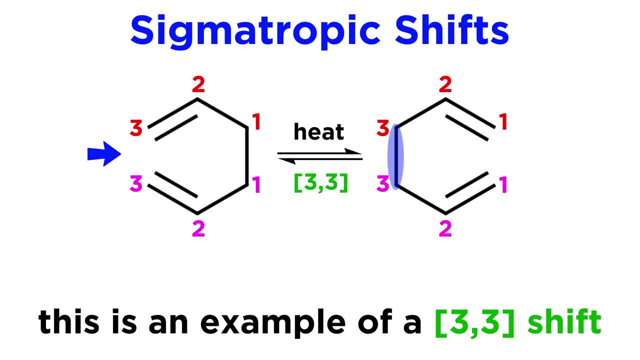 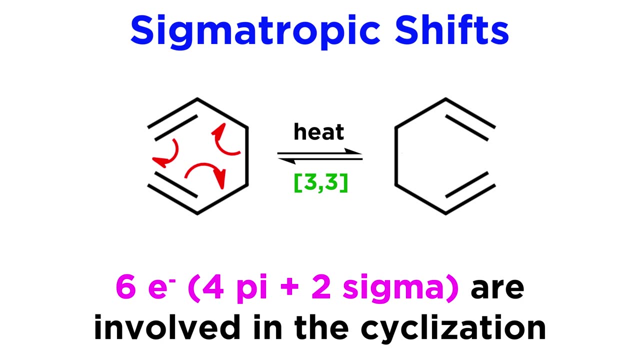 between carbon 1 and carbon 1 is broken and the new sigma bond is between carbon 3 and carbon 3.. That's why this is called a 3-hexadiene. Once again, the number of electrons involved in the cyclization is 6,, 4 pi and 2 sigma. 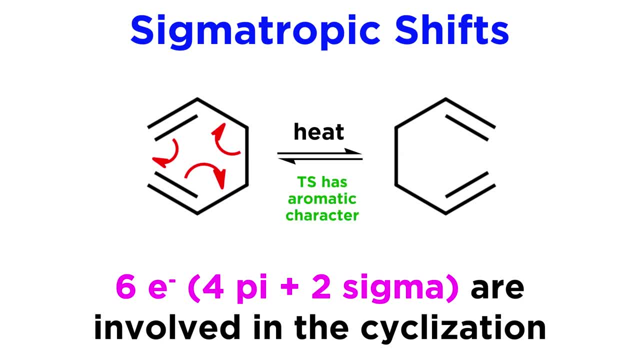 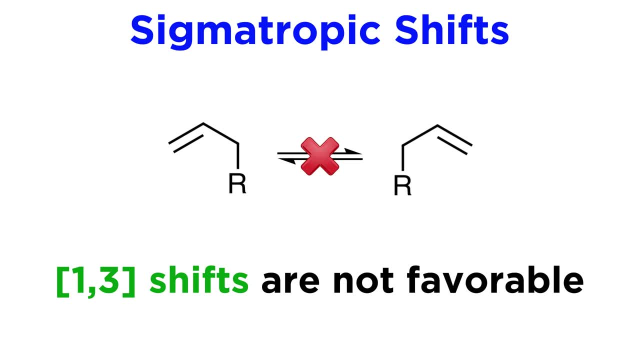 which is why this reaction is allowed, as the transition state can be thought of as aromatic in character and therefore stabilized. To get a sense of what is not permitted in this context, take a look at an example of what would be considered a 1,3 shift. 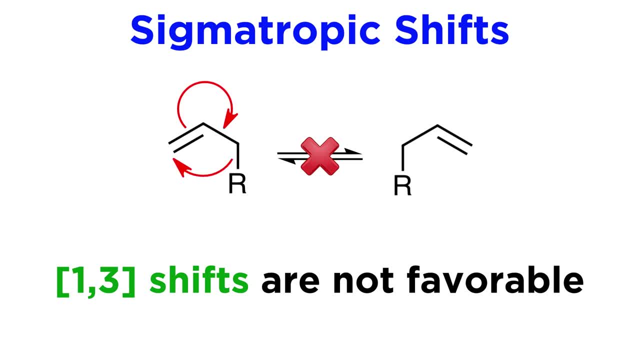 This would essentially entail the migration of this alkyl group over to the other terminal carbon. in this allylic system with two sigma and two pi electrons involved in the shift, Numbering the alkyl group 1, and then 1 through 3 for the other fragment, we can see how it would be numbered this way. 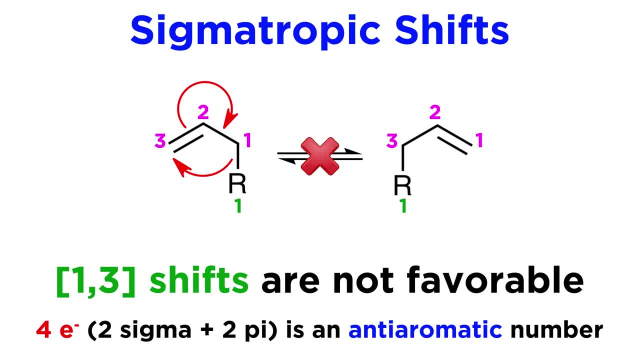 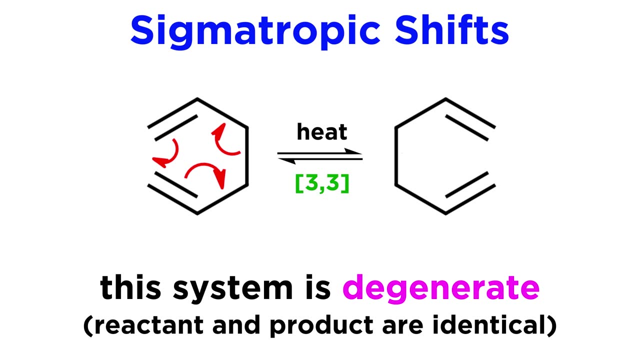 But 4 is an anti-aromatic number, so this is not a favorable process and indeed a shift of this kind is rarely observed. Returning to the 3,3 example, this simplest system here can be said to be degenerate, That is to say the product is the same as the starting material. 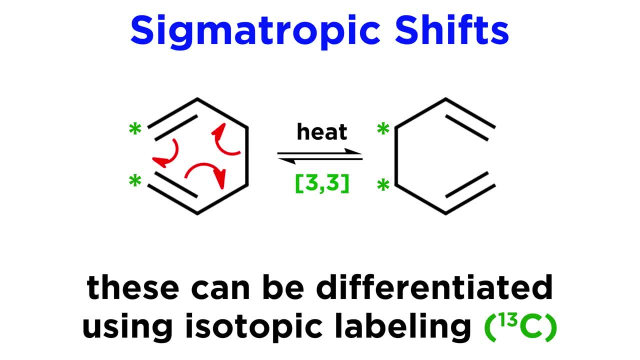 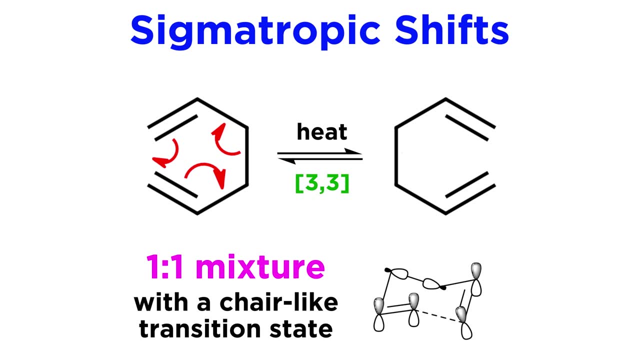 and can only be differentiated if we were to incorporate isotopic labeling, such as if the asterisks we used earlier implied carbon-13 nuclides. Because this system is degenerate, we can expect a one-to-one mixture with chair-like transition states as it shifts from one form to the other. 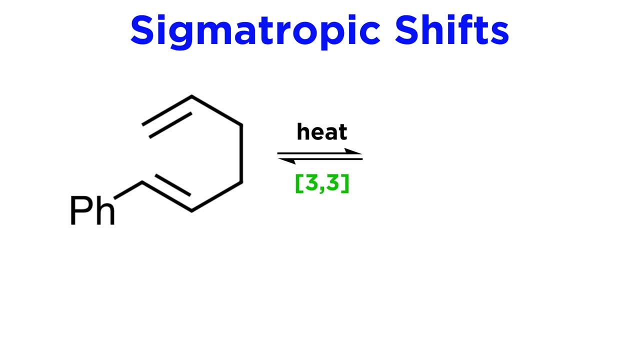 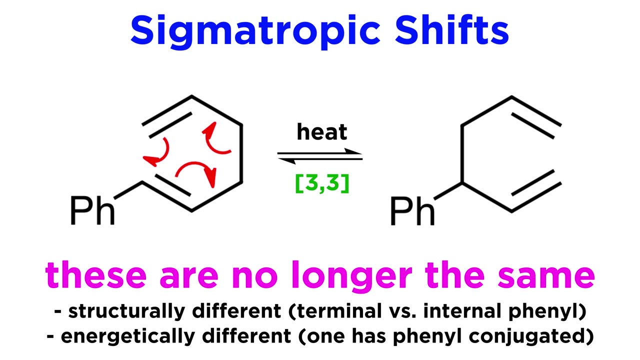 We can begin to see a discrepancy in the two structures by adding substituents. For example, let's put a phenyl group on this terminal carbon. If the shift were to occur, the phenyl group would be on an internal carbon. so these structures are no longer the same. They are also not of the same energy, because we can. 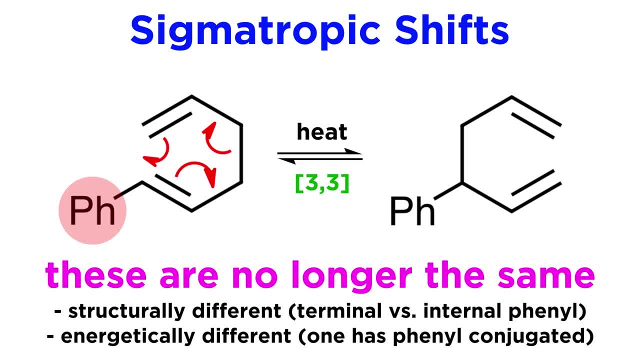 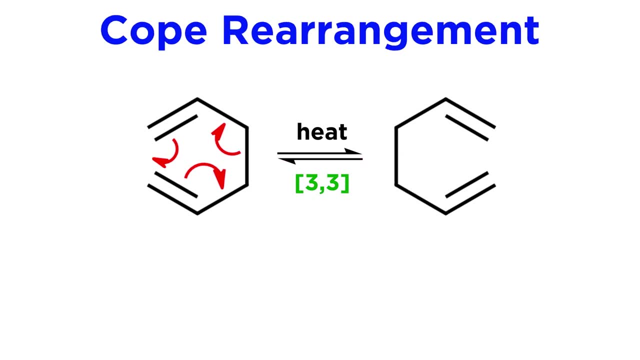 see that in the first structure one of the pi bonds is conjugated with the phenyl group, whereas in the other it is not. So this is where we can begin to see the equilibrium shift more over the other. These examples we have just examined. 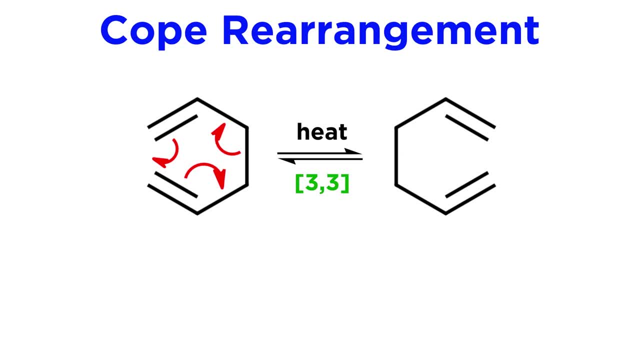 can also be referred to as the cope rearrangement. These usually require temperatures of around 200 degrees Celsius to proceed. One may question the synthetic utility of this technique, as even when an equilibrium prefers one form over another, there is still the disadvantage of low. 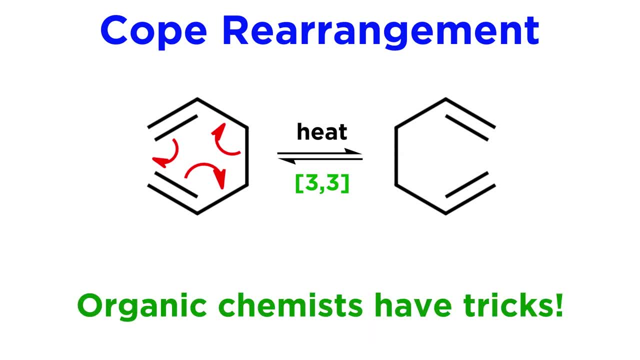 yield and the necessity of separating from starting material, But organic chemists have come up with a way to do this. One approach is to generate some starting material that is dramatically more unstable than the product of the sigmatropic shift, and one way to do this. 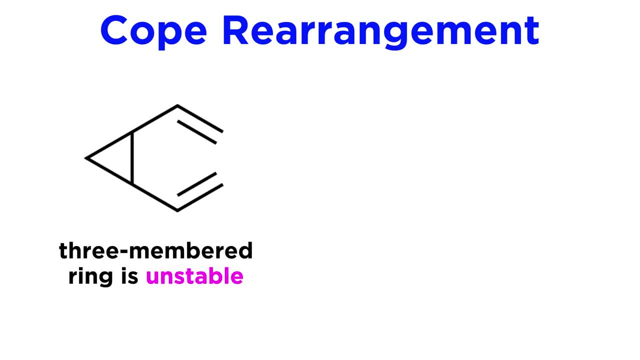 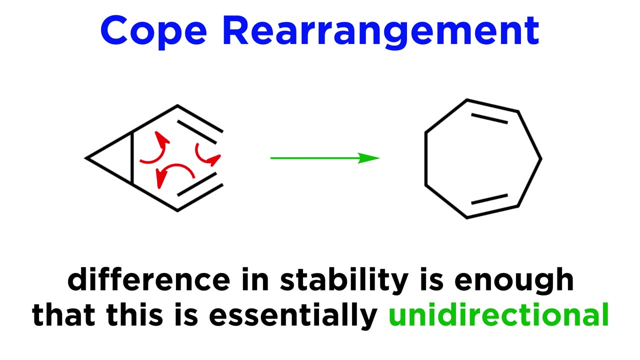 is to incorporate ring strain. For example, consider this structure with a cyclopropane ring. In carrying out the reaction, the three-membered ring is cleaved and a seven-membered ring is formed. The difference in stability is so extreme that we can consider this to be essentially 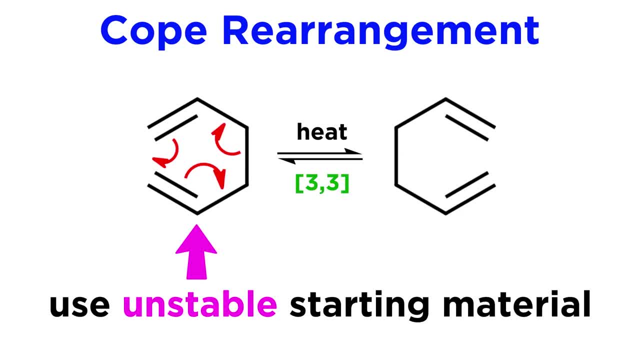 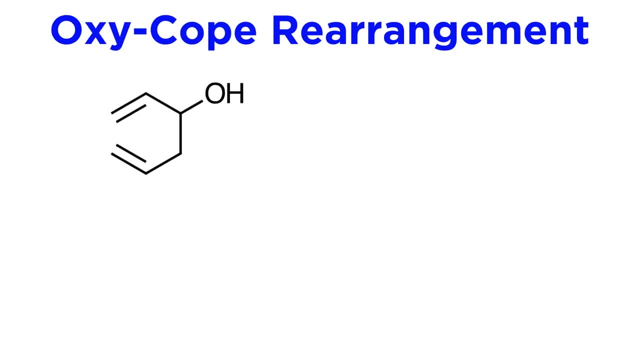 unidirectional. Similarly, instead of destabilizing the reactant, we can also stabilize the product. Take this substrate, for example: with a hydroxyl in this position, If the shift is carried out, an enol will result which, as we know, will rapidly tautomerize to. 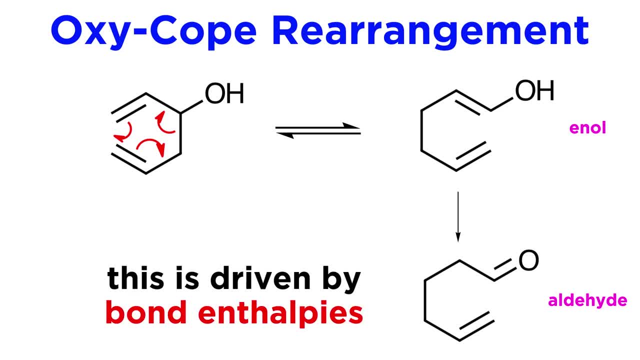 give the carbonyl, in this case an aldehyde. Here, bond enthalpies are responsible for the stability of the product, with the carbon-oxygen double bond being especially strong. This modification of the Cope rearrangement is called the oxy-Cope rearrangement. 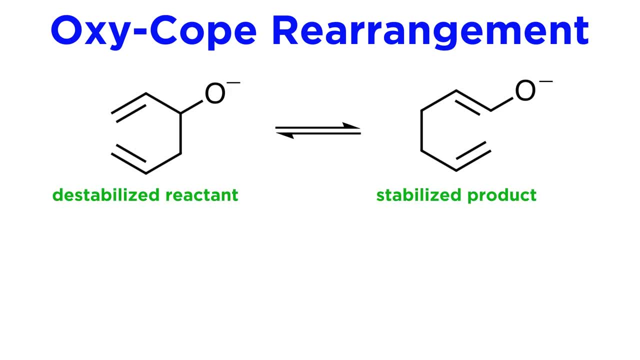 Now, if we combine these approaches, both destabilizing the starting material and stabilizing the product, the reaction becomes favorable enough to occur even at room temperature. Consider the same starting material as the previous example, but with an oxyanion instead of a hydroxyl. This is unstable, as the anion is localized on the oxygen After the 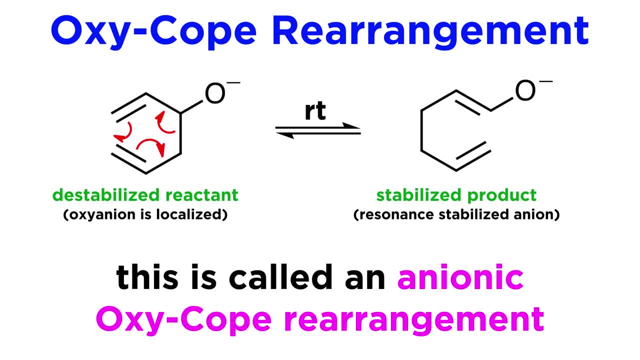 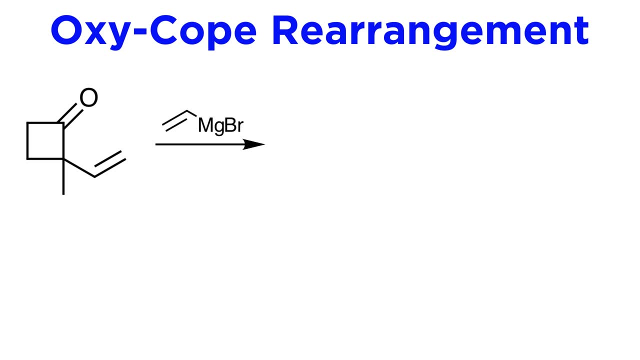 shift the anion, is resonance stabilized. We would call this the anionic oxy-Cope rearrangement, and this technique is prevalent in synthesis. To see an example of its application, consider this: substituted cyclobutanone Treatment with a vinyl Grignard reagent will produce this magnesium alkoxide intermediate. 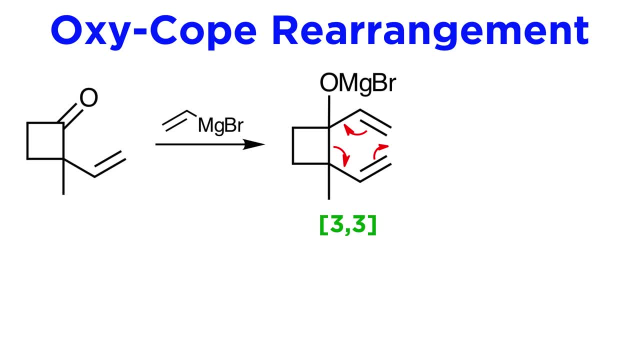 which we can quickly see, is capable of a 3,3-sigmatropic shift via oxy-Cope rearrangement, But this is not the case for any of the other techniques we discussed in this video. Breaking this sigma bond has the ramification of cleaving the four-membered ring and producing an eight-membered. 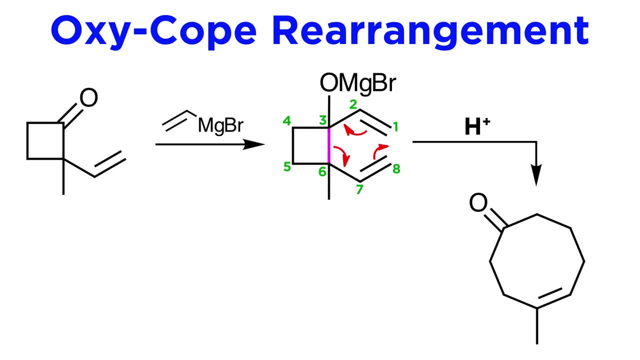 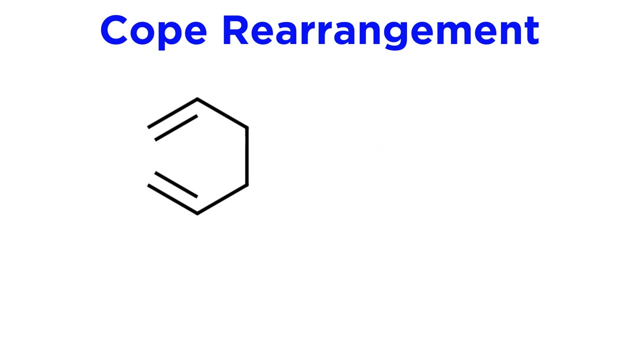 ring and acidic workup will produce the enol which will tautomerize to give the ketone. And that leaves us with this cyclooctenone, the product of ring expansion through the oxy-cope rearrangement. Let's make one more modification on the cope rearrangement. We can replace one of 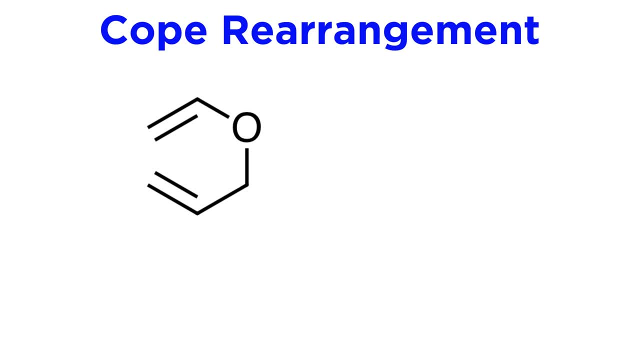 the carbon atoms, with an oxygen atom, perhaps on carbon three to give this ether. Now let's allow the three-three shift to take place and, as we can see, we are left with an aldehyde. As we might imagine, bond enthalpies dictate that this equilibrium will lie heavily to the right. 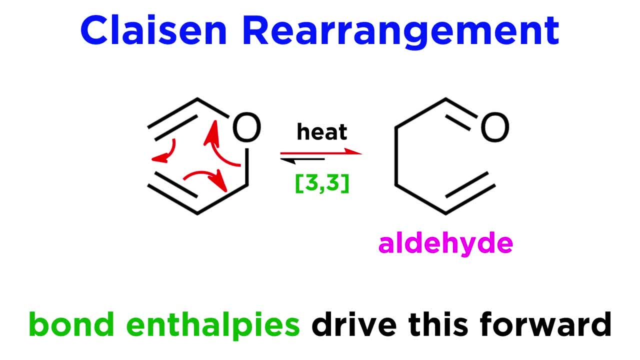 favoring the stable carbonyl. This variation is called the Claisen rearrangement and it is a great way to synthesize gamma-delta unsaturated carbonyl compounds, where we are calculating the carbon atoms with an oxygen atom, perhaps on carbon three to give this ether. 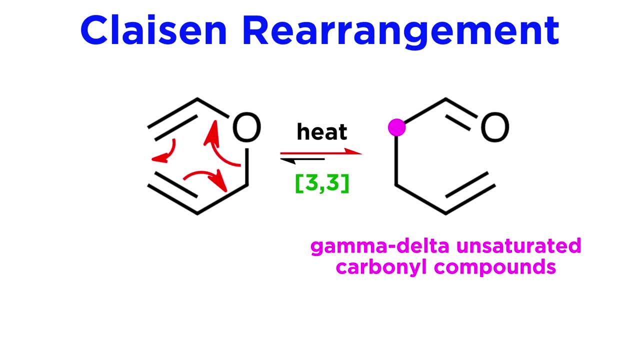 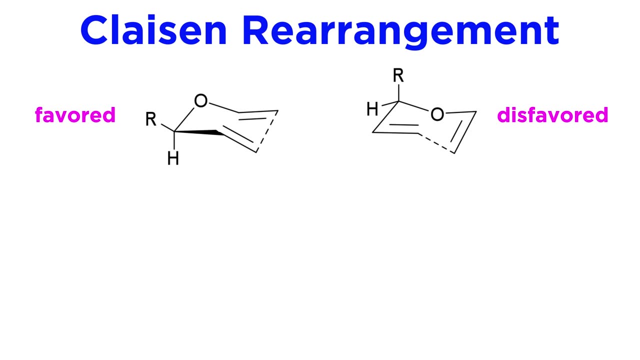 Counting up the Greek alphabet from the carbonyl carbon, alpha, beta, gamma, delta with the other pi bond in the product sitting between the gamma and delta positions For Claisen rearrangements where substituents are present, given the chair-like transition state. 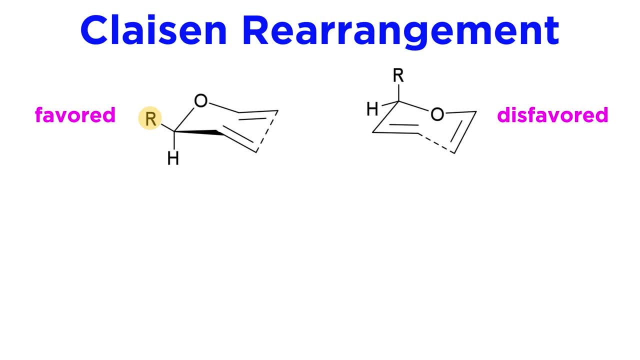 substituents will prefer to occupy pseudo-equatorial positions rather than pseudo-axial, and the olefin products will tend to form with E configuration rather than Z. The interesting thing about this rearrangement is that the driving force of carbonyl formation 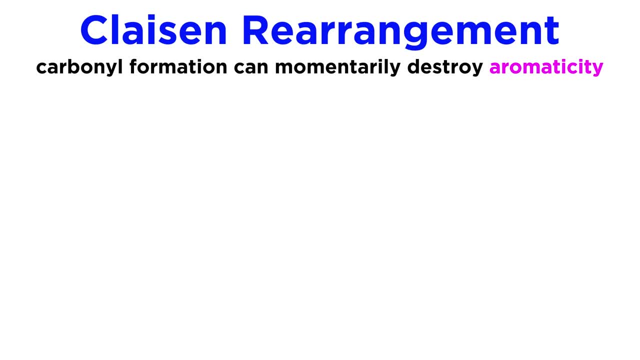 is even enough to momentarily destroy aromaticity. Consider this starting material Upon heating. the three-three shift will take place, despite the fact that it requires breaking the aromaticity of this benzene ring. The reason this is possible is that tautomerization can then take place. 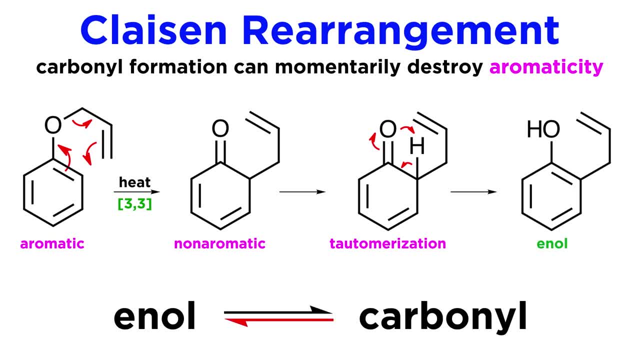 to yield the enol, which is the opposite direction we're looking at. So let's look at the three-three shift. The three-three shift will take place despite the fact that it requires breaking the aromaticity of this benzene ring.